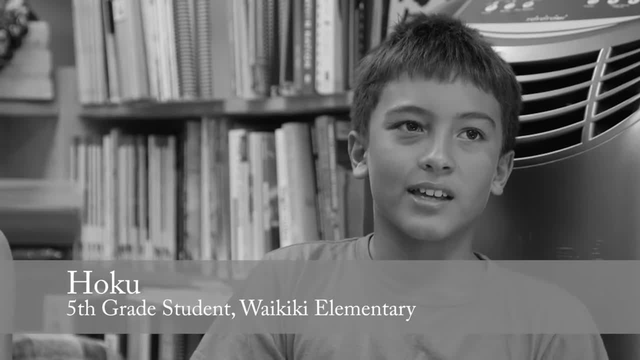 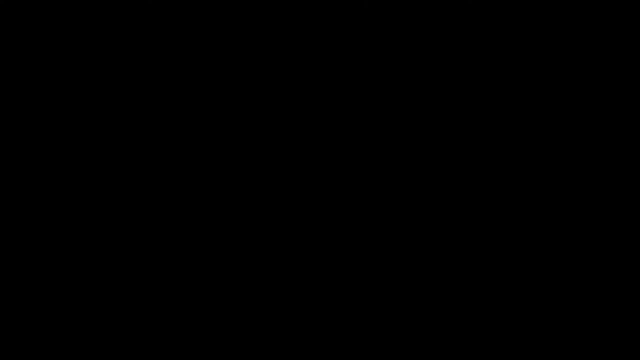 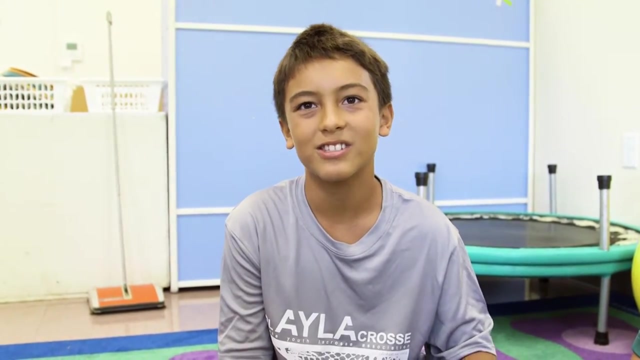 Before I started P4C, I would like get all mad at my friends and try to punch them and stuff. When I'm mad and I come back to class, I just want to scream At a P4C. I can turn that screaming into words. 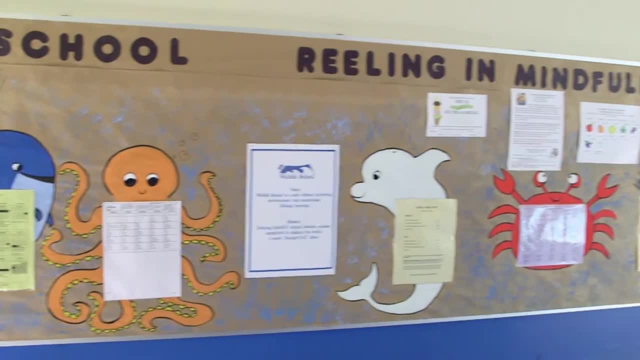 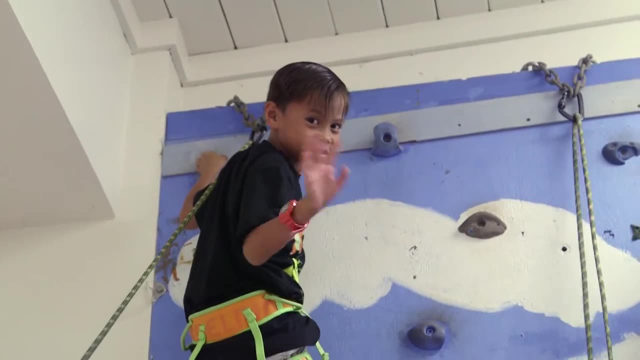 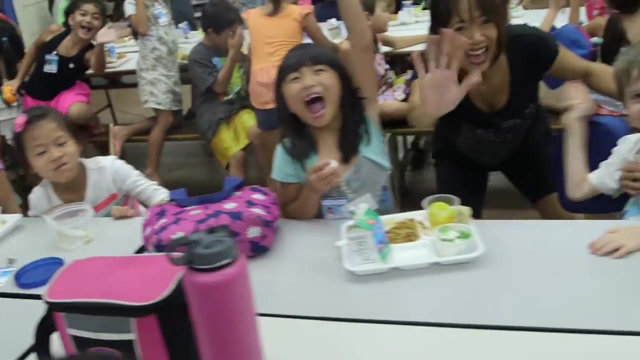 We've had two teachers of the year. We've gotten blue ribbon awards twice, The first to be certified as a mindful learning center school. There's a big surge of people who want to come and put their children into our school because they believe in the kinds of things we're doing here. 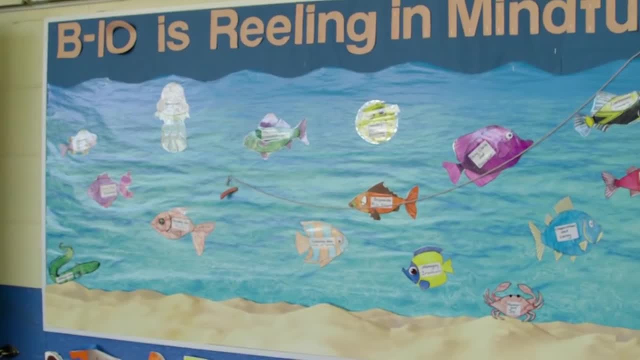 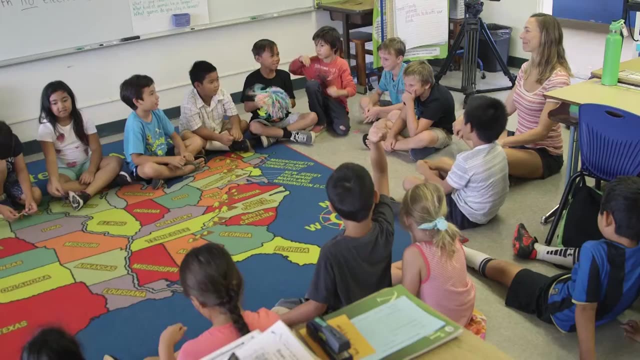 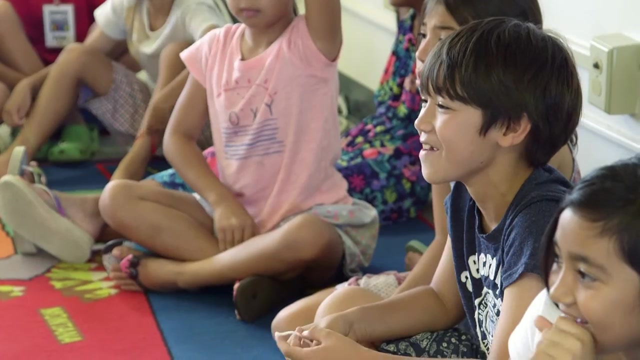 Through this program- Philosophy for Children program- we were able to achieve the goal of helping our kids become better thinkers. When I think of P4C, I think about creating a particular kind of place where people genuinely listen to each other, and listen to each other with care. 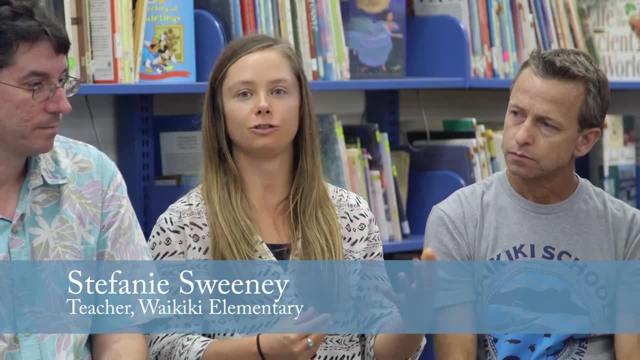 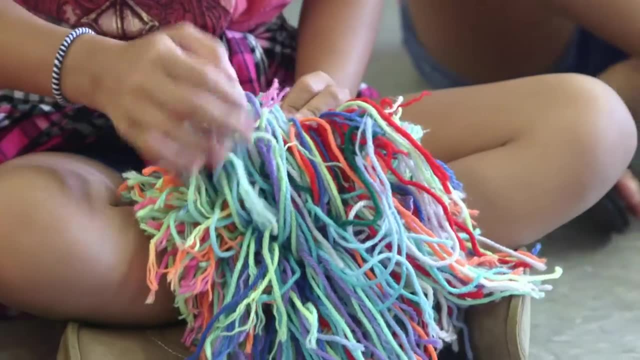 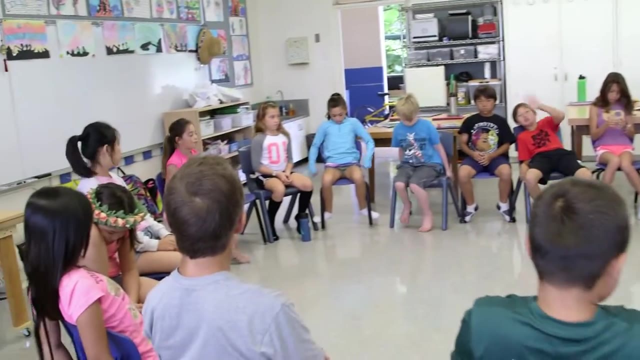 P4C gives students a chance to ask their own questions. They get to choose the subject of their discussion. During the discussion, the person that speaks has a ball of some sort. This is the community ball. The community ball goes from one person to another, and the choice of who it goes to is once again chosen by the student. 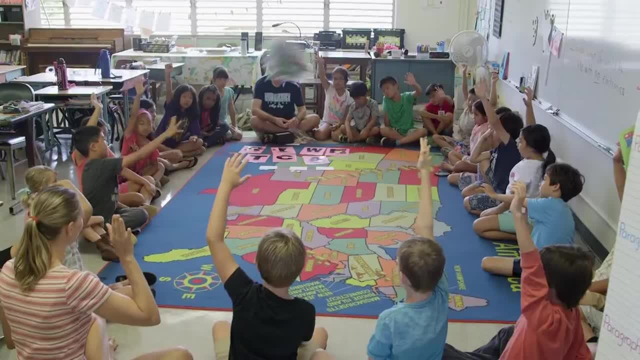 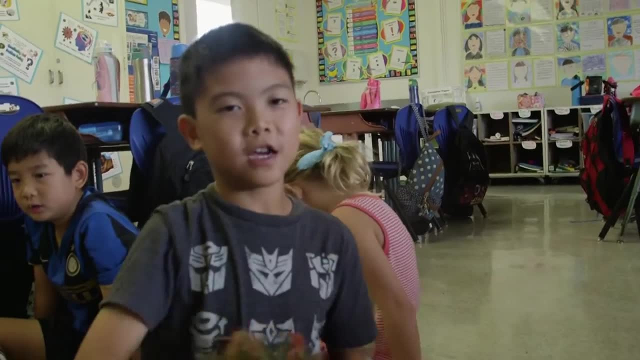 So the idea of we're thinking interdependently and we're going to come up with ideas that we wouldn't be able to come up with on our own. Do you like P4C? and why I like P4C? because you get to talk about interesting topics. 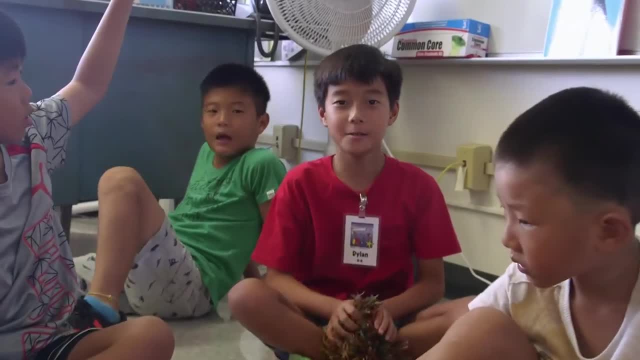 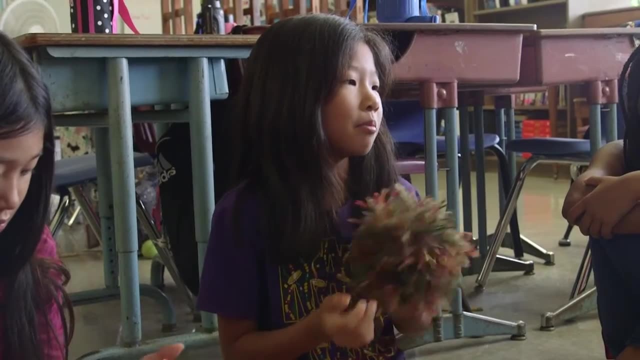 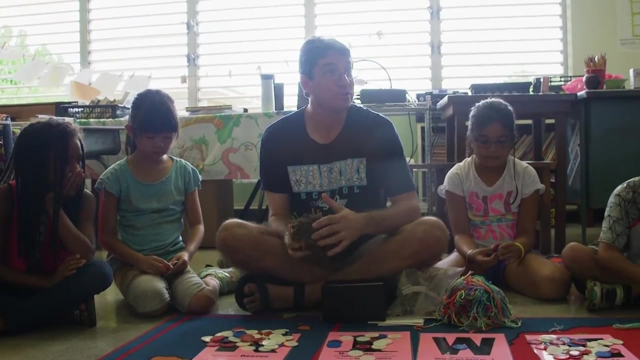 Laugh, Pop up, Fill in, You get to really think and exercise your brain. Curate, Teach. It stretches out your mind. Isabella, I don't like P4C, I love P4C. Thank you, boys and girls. 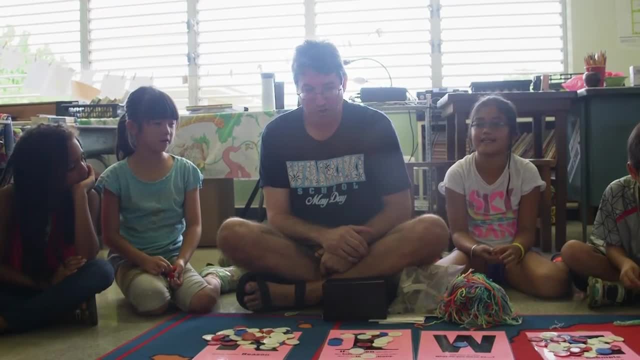 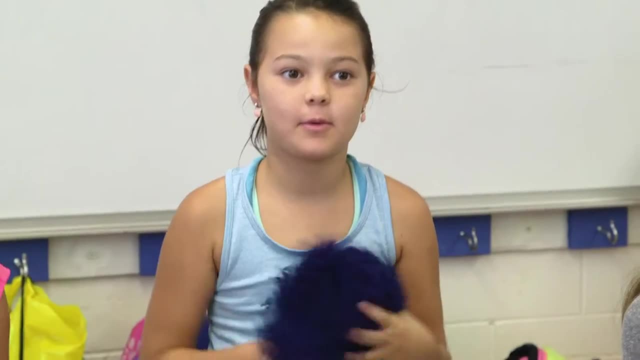 It's fun doing P4C, Mr Toby, As always, And look at all the GoodFingers tools, And thank you to Heidi and Liam. They're the ones who put all these down. I end up letting them drive the curriculum in a lot of ways. 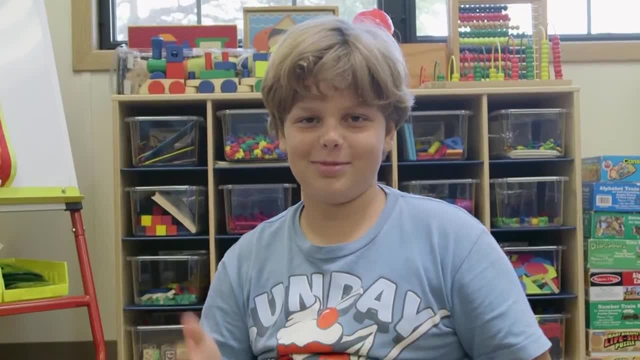 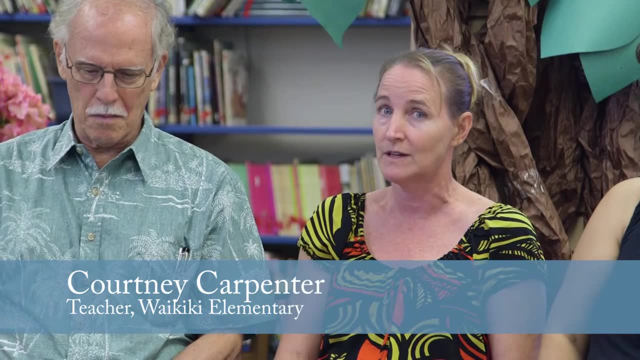 I mean I still have to cover certain things, but I know that they're going to tell me what they need, because they're able to communicate what they need, because they're used to speaking up and asking questions And through these questions I'm able to figure out what specifics I need to teach.